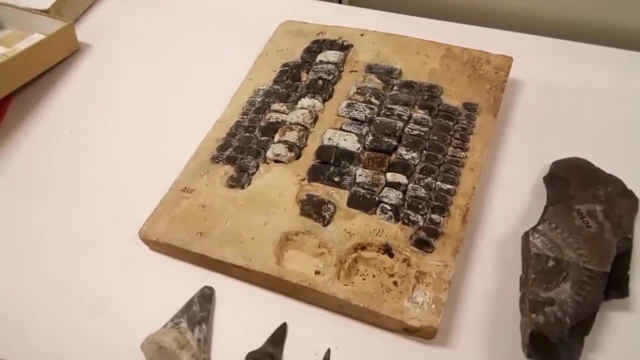 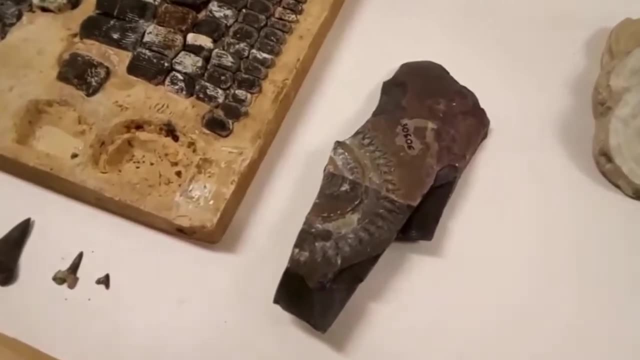 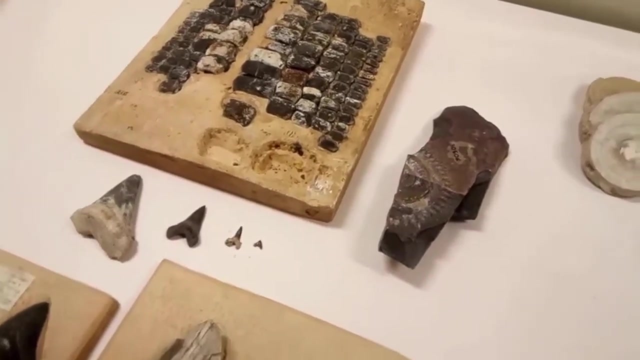 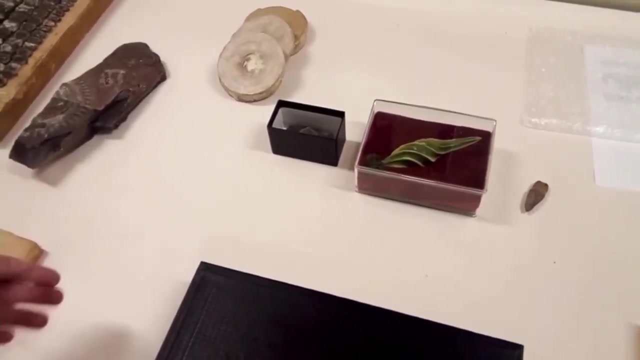 call pavement tooth sharks, which were grinding up things like mollusks. And then we have a shark that had a really unusual spiral jaw And we actually don't really understand how that was used or why it had it. Typically, teeth are the first and sometimes only parts of the body that 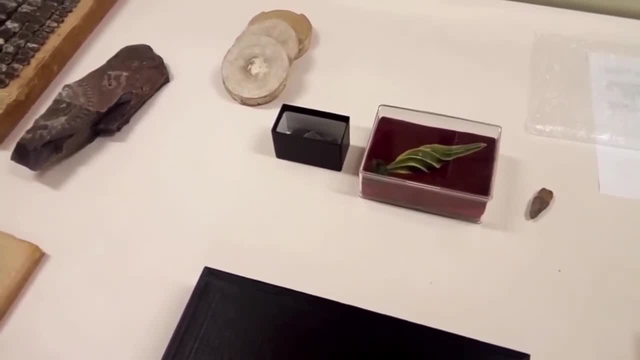 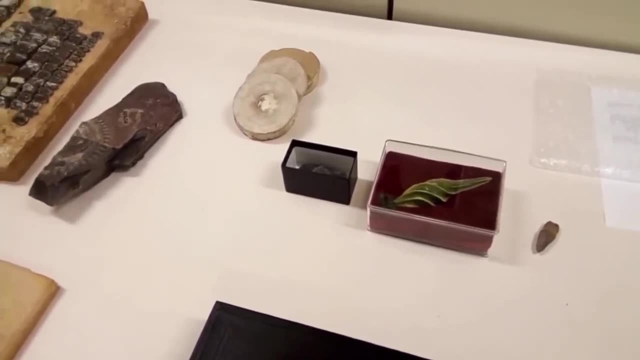 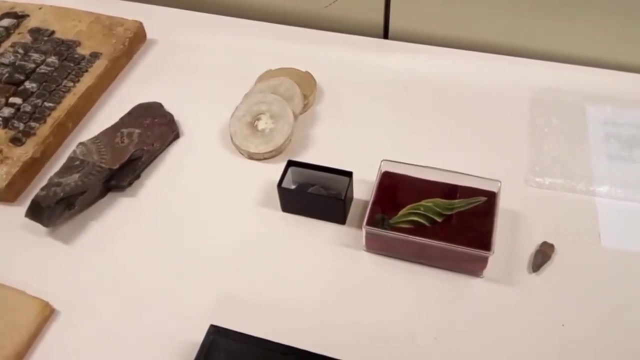 are fossilized because they are covered with enamel, which is the hardest substance in an organism's body. But sometimes we will get parts of the skeleton or even trace fossils which aren't parts of the body itself but evidence that the animal was there. So here we have some really unusual 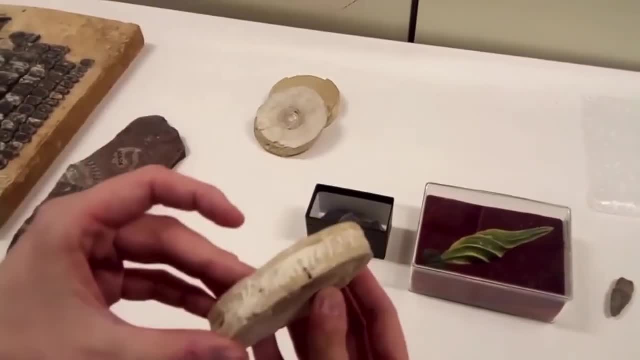 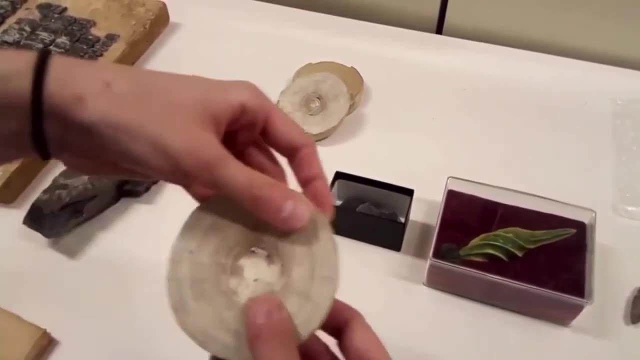 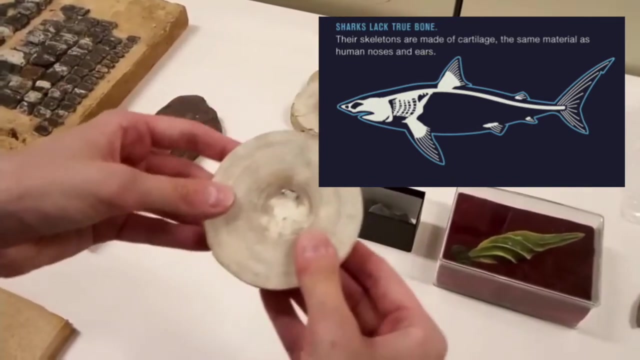 specimens of shark vertebrae. They have been compressed so they used to be wider Body. fossils are really unusual because sharks have a cartilaginous skeleton, So their skeleton is actually not made of bone like ours is and like mini fish, And cartilage can't fossilize. 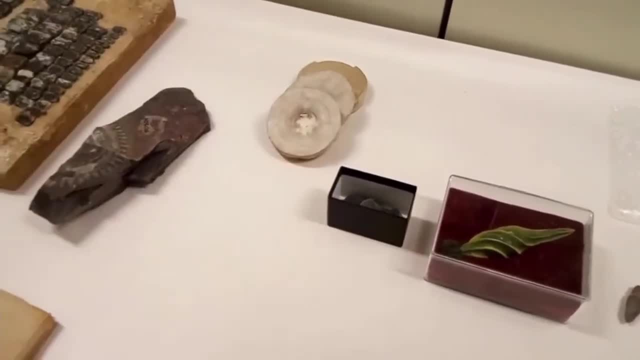 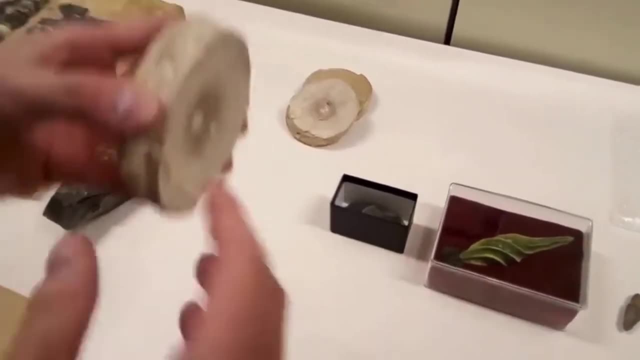 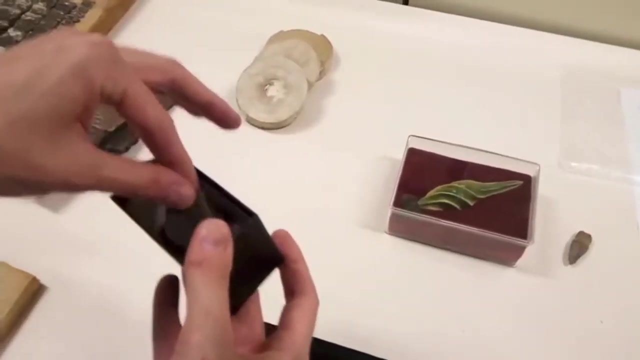 as well as bone. So typically the only thing that's left from a shark are their teeth, But we do have many specimens here at KU that preserve parts of its body. We also have some trace fossils from sharks. This is an example of a very rare one. 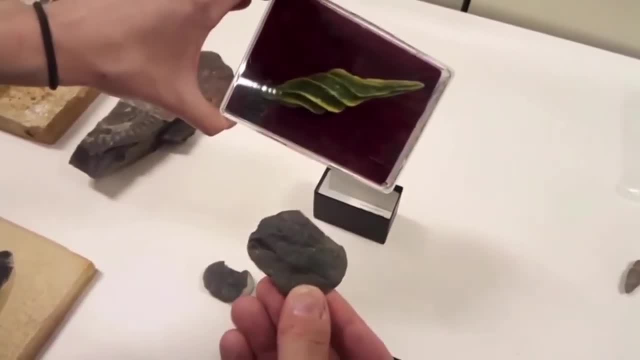 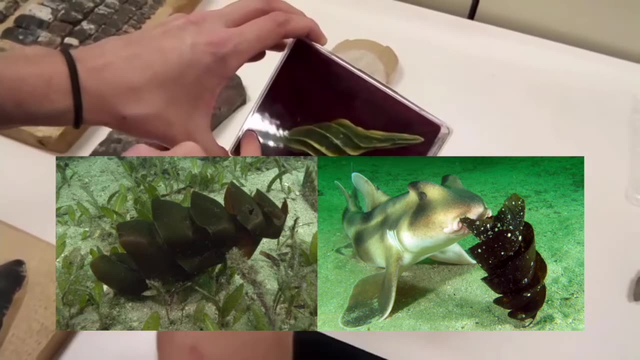 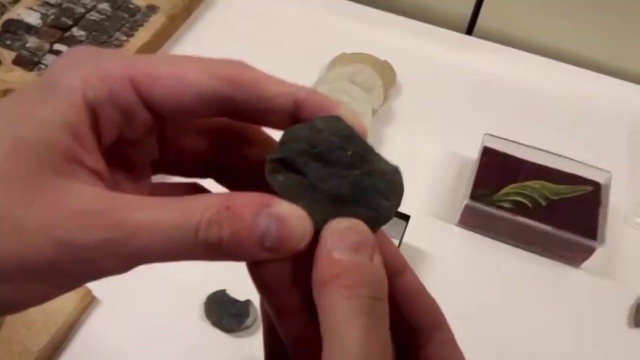 You can see here that we have a model. This is an egg case from a shark, So you can see that it's bulbous in the center, It tapers out toward the end and it has a spiral pattern around the outside. It might be difficult to see, but this is a nodule from here in Douglas. 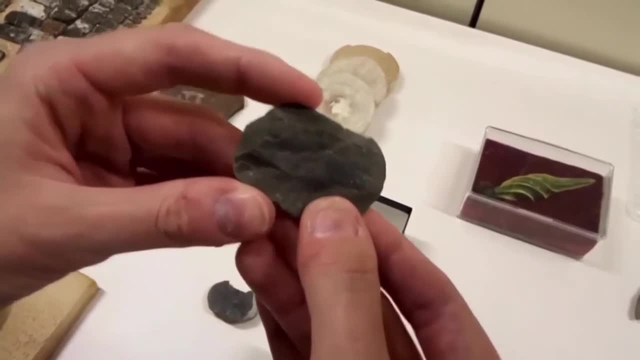 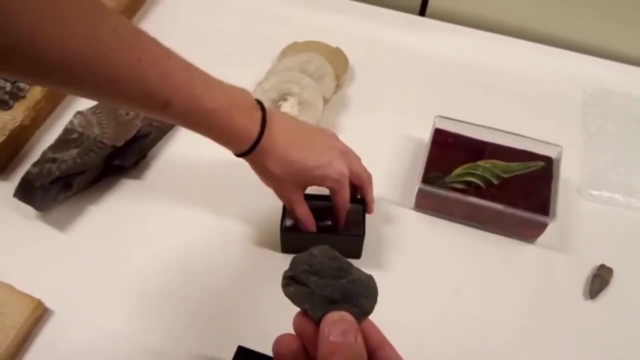 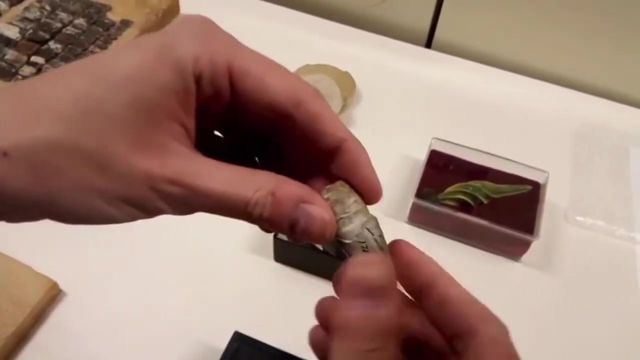 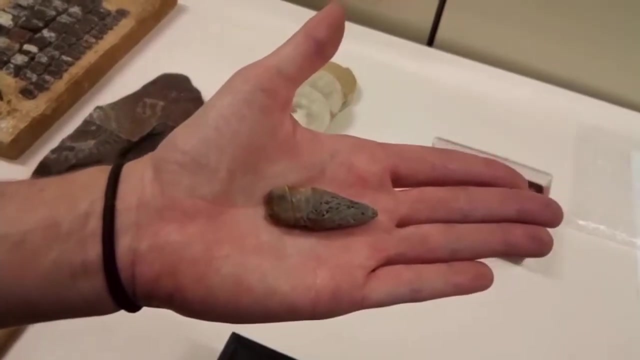 County where Lawrence is, And this is a fossilized egg case from a shark that dates all the way back to the Pennsylvanian And we also in the collection have many coprolites from fishes. So a coprolite is a fossilized piece of remains from inside the intestines in the colon of an 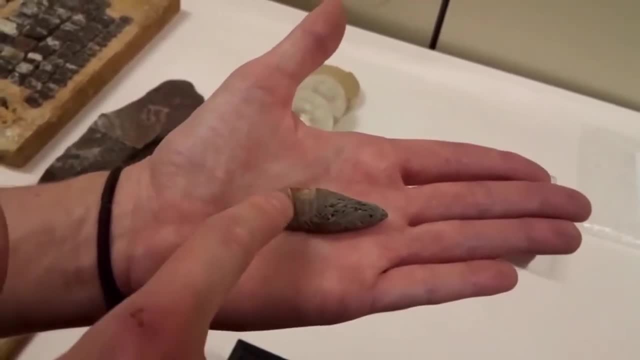 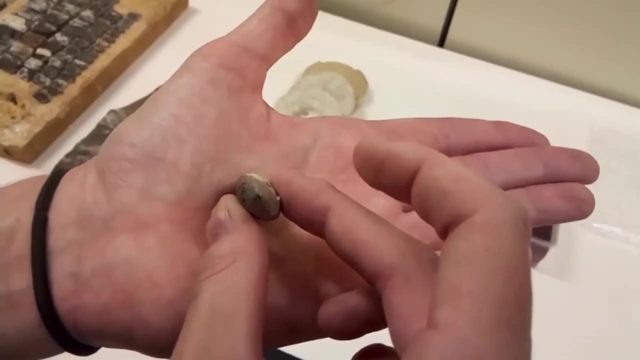 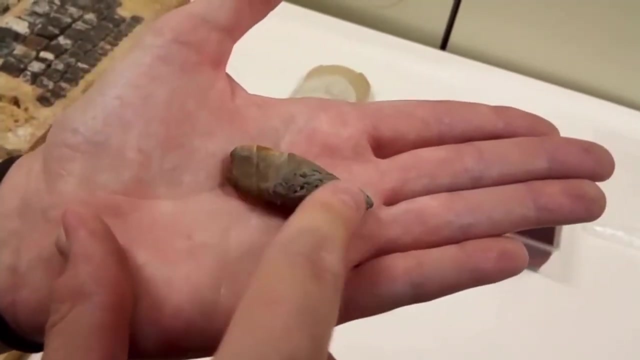 animal. You can see that it has ridges here that represent the ridges inside the intestine of this fish. It tapers with the conical end which is where it was pinched off, And this one even has tiny bones which are the black specks of probably the other fish that it. 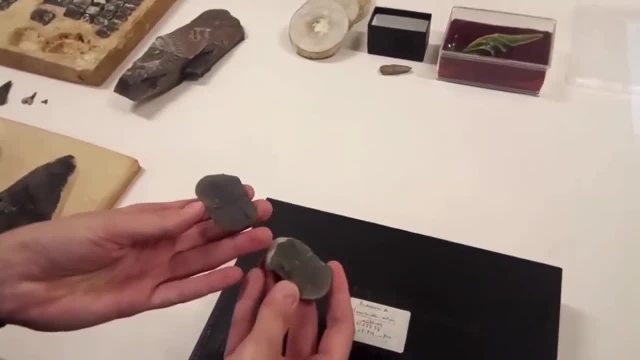 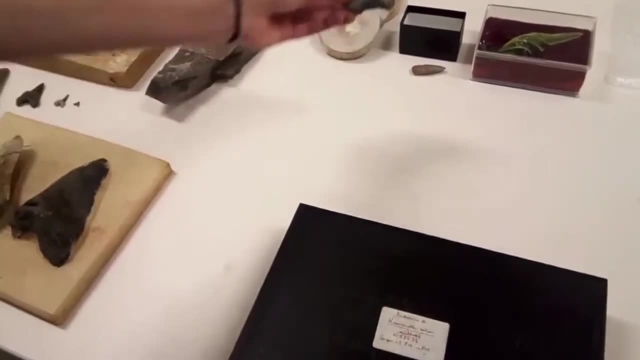 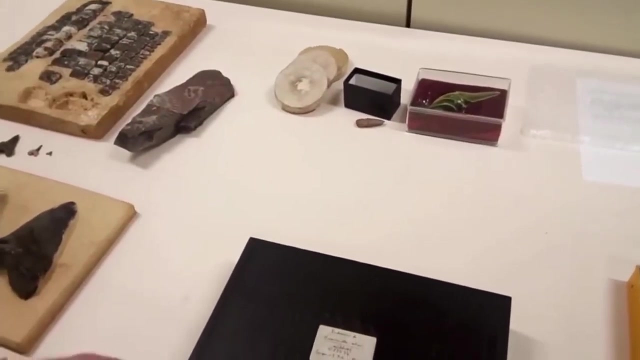 was eating. Like the egg case that I just talked about. it was found inside a nodule Here in Douglas County, Kansas. We have hundreds of nodules just like that in the collection And that's the only one that has an egg case inside, but the others have parts of the skull and 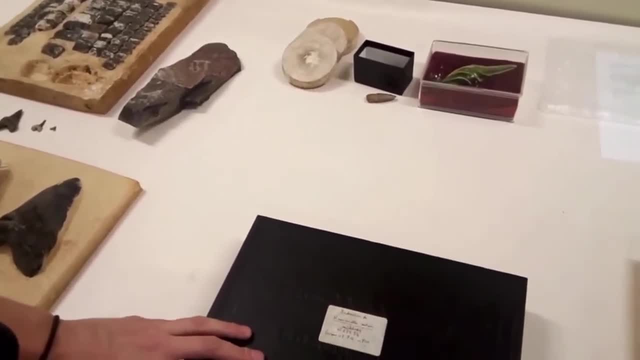 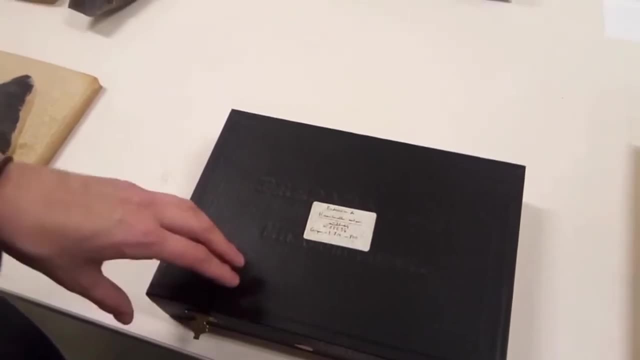 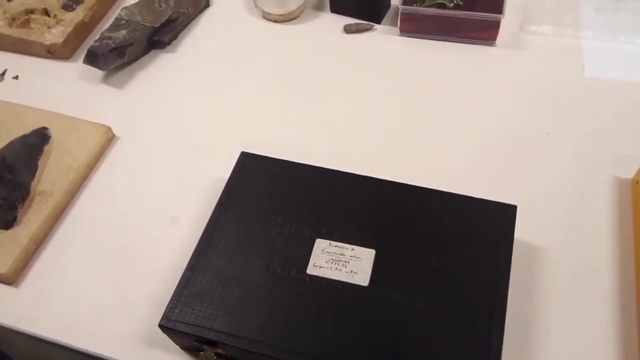 sometimes brain cases from a different kind of bony fish. There was a group in France in the 70s and 80s that studied those nodules from our collection. We shipped hundreds of them to France. They studied them. Some students wrote dissertations about them. 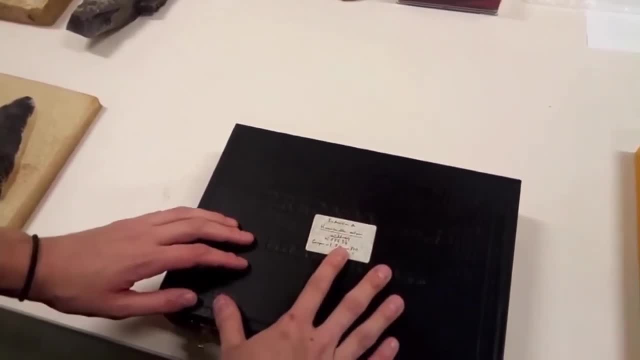 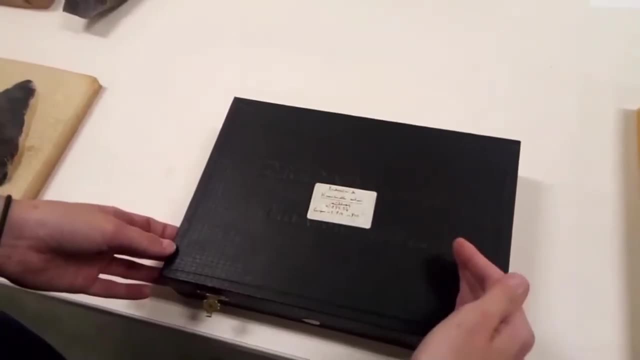 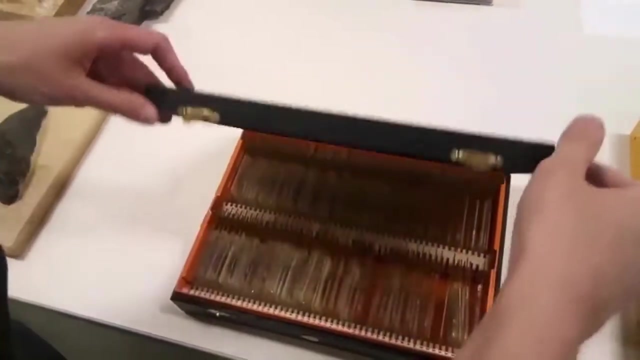 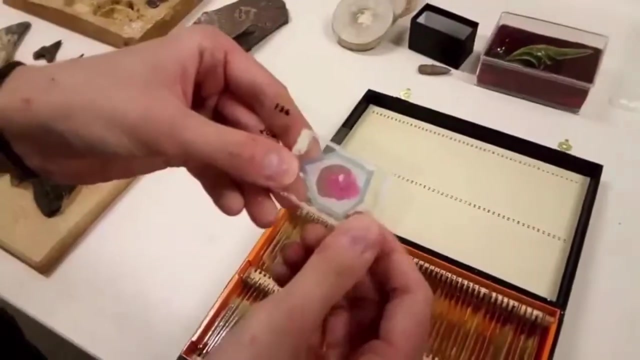 And for a couple of specimens that were interesting. they took slides of those specimens. Essentially, they cut them up into slices and encased each slice in a separate slide. So this specimen total had 1400 slides. They did this so that they could see the internal structure of the specimen. 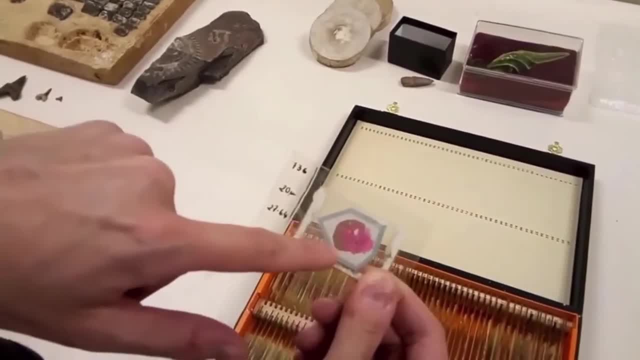 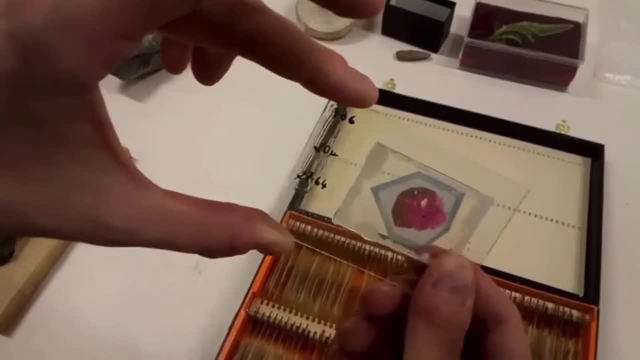 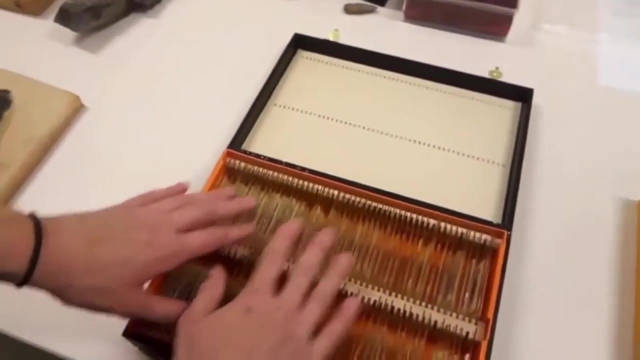 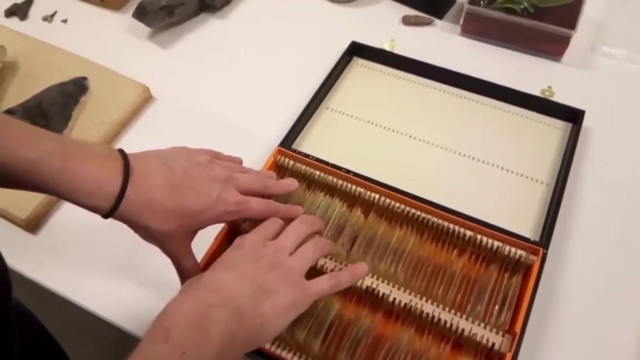 This happens to be a brain case from that bony fish And you can see the red portion that's highlighted or dyed. So, like I said, they would do this to see the internal structure because previously they could only see the external portion of that brain case, And sometimes they would also do it to reconstruct. things in 3D if the specimen had been cut out for some reason, especially if the species had been cut out for some reason. So that's just a quick example of what happens when you want to see the most specific specimen. Some specimens actually take a little bit longer. 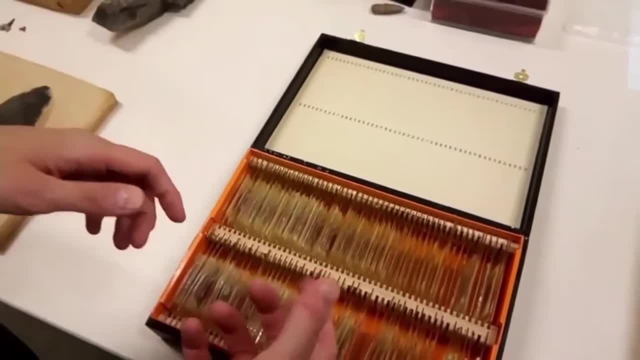 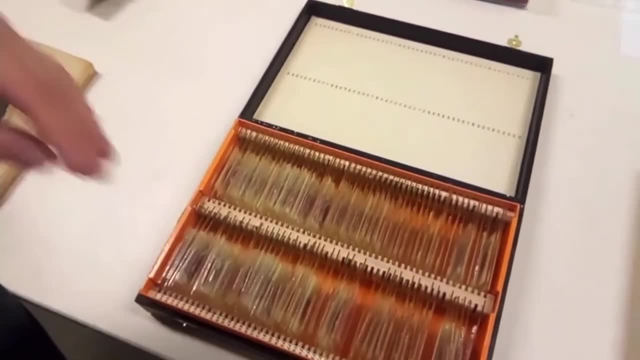 Some specimens actually take a little bit longer- had been found compressed or flattened. Today we do the same process, but we don't have to cut up the specimen or use any destructive technique like this. We would CT scan a specimen and the computer will take photos. 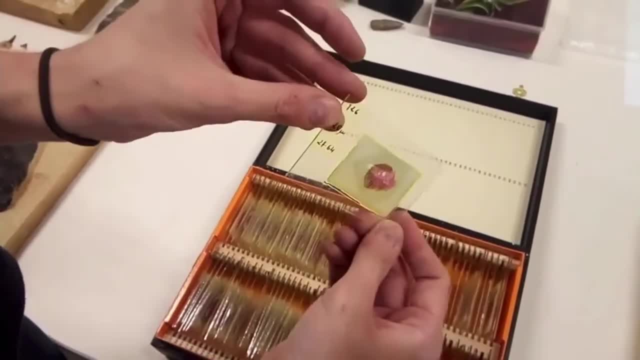 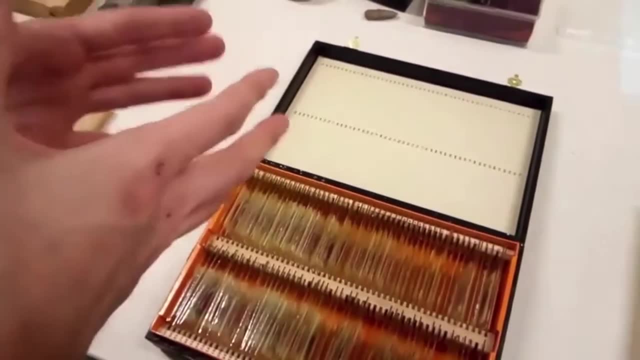 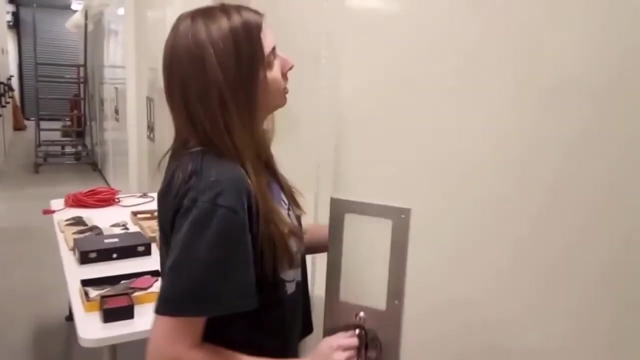 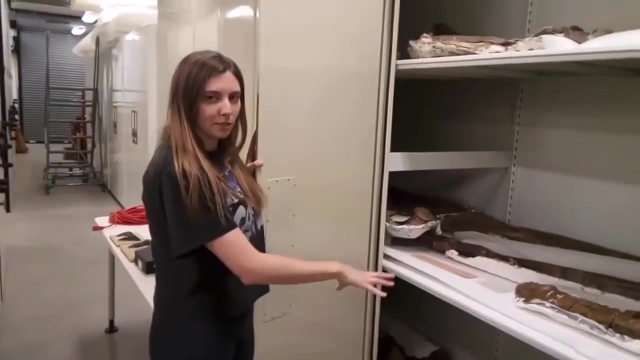 that represent each of these physical slides. So we end up with slices and a series of photographs that we can then put together to reconstruct the specimen or see the internal structure. So these are all jacketed dinosaur bones from the late Cretaceous of New Mexico. 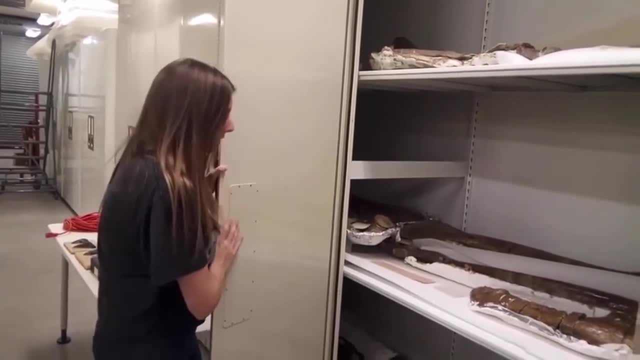 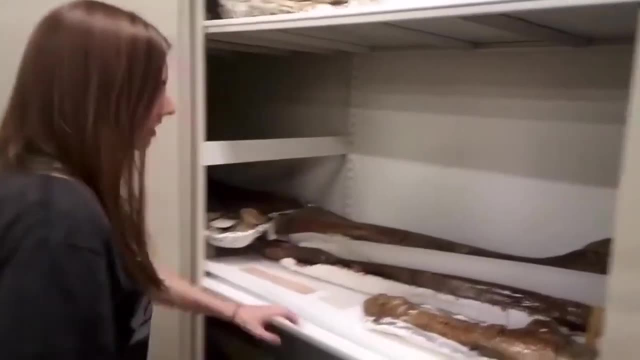 from the Fruitland-Kirtland Formation. It looks like we've got a femur part of a jaw and a few other big limb bones. This is a project and a cyclops is a cyclops. This is a cyclops. 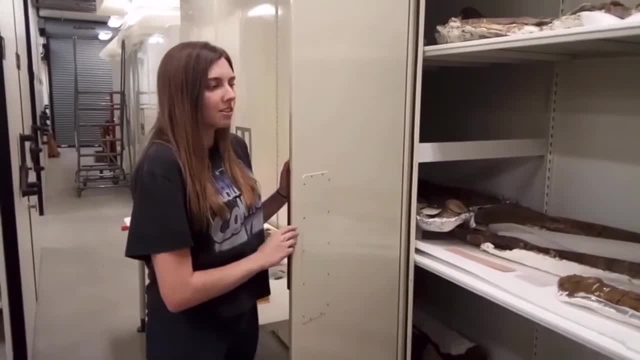 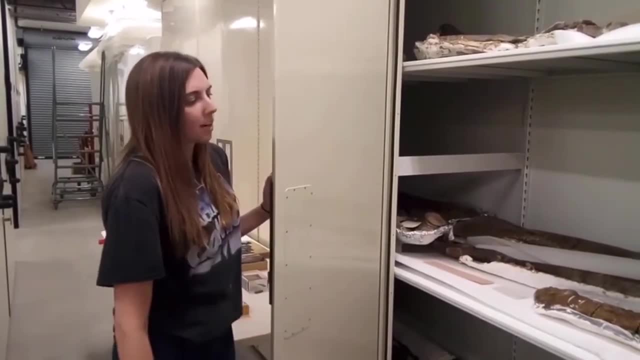 This is a site that was excavated by KU teams from the 60s, throughout the 80s to 90s, And then we abandoned that project. It has recently been picked up by a team at the Denver Museum of Nature and Science. 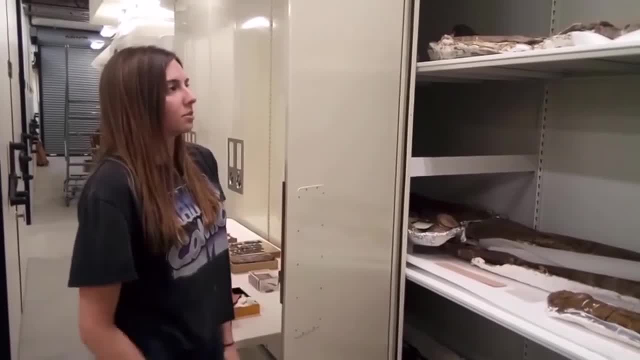 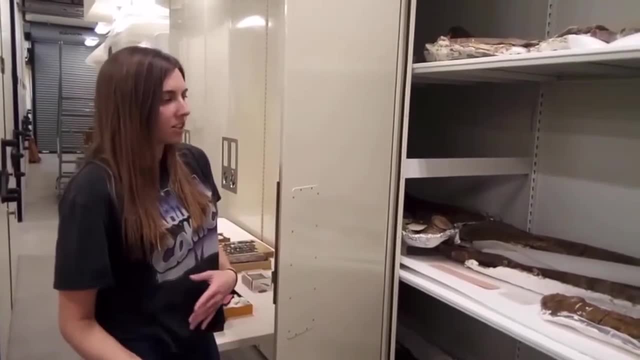 So some of their people have come to look at this collection and sort of see what we already have And as they're working out in the field collecting more from this site for their collection, they're going to continue to come back here, work with us and look more at this collection. 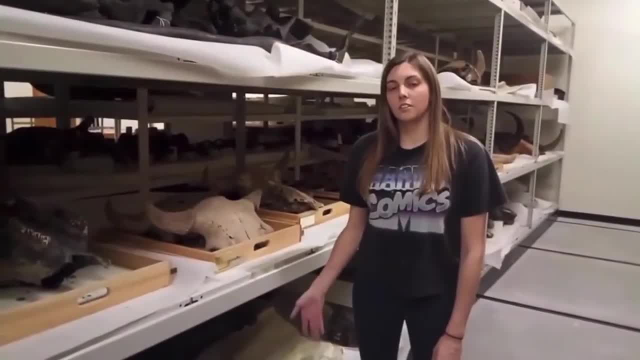 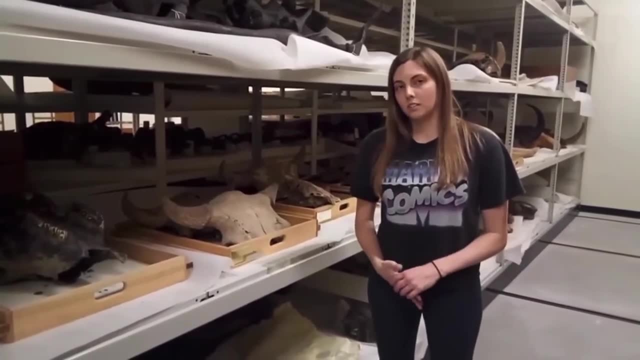 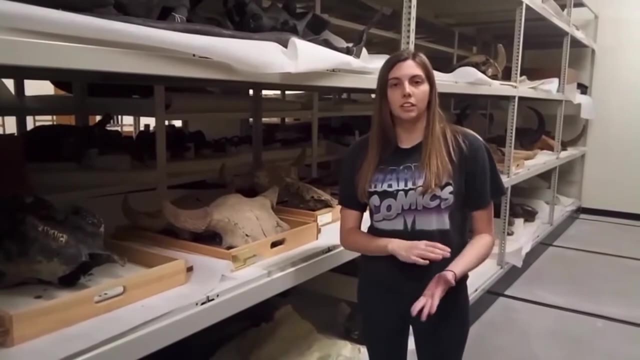 to compare what we found. Another large part of our collection are Pleistocene mammals, mainly bison, because they were really numerous during the Pleistocene, But we have collections both from a site in Wyoming called Natural Trap Cave that I'll talk more about later. 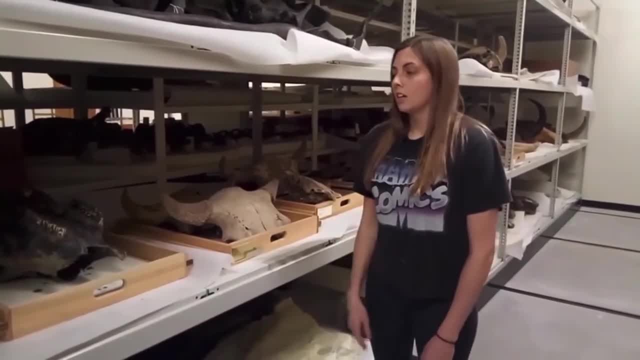 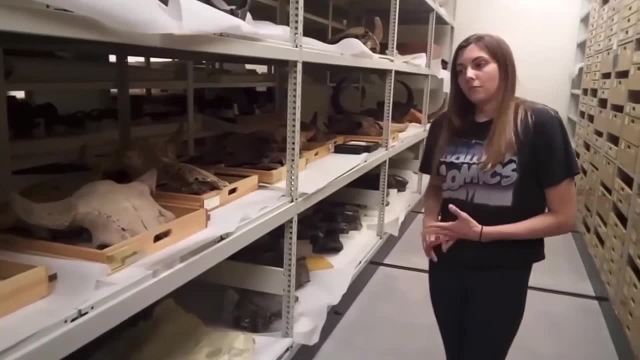 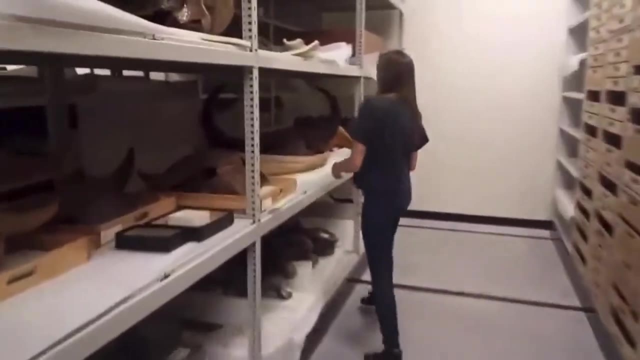 and also the Kansas River, right here in town. You can see that we have, even within bison, a large diversity of both male and female, juvenile and adult, and many different species, The biggest of which is this, which is a single horn. 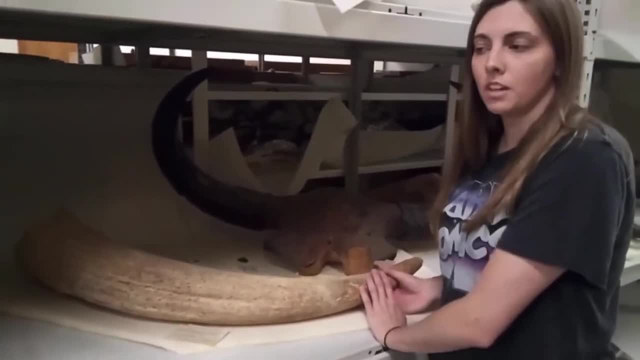 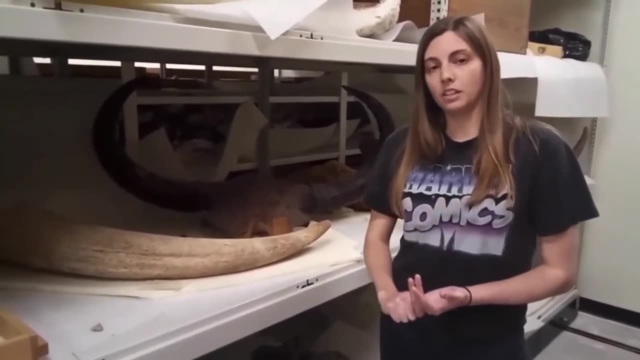 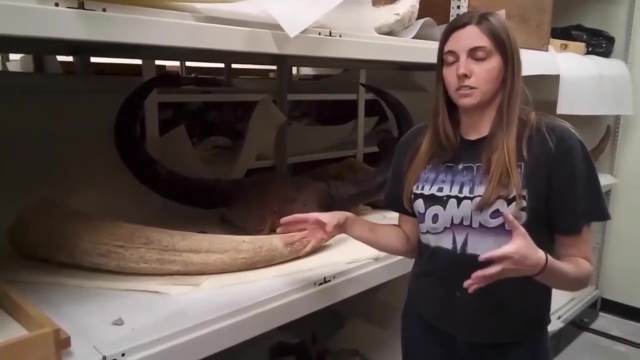 from a bison called bison latifrons. Many people come to KU to study our Pleistocene collection, One because it's so big And two because we have many representatives from different sites So they can test specimens from different sites.